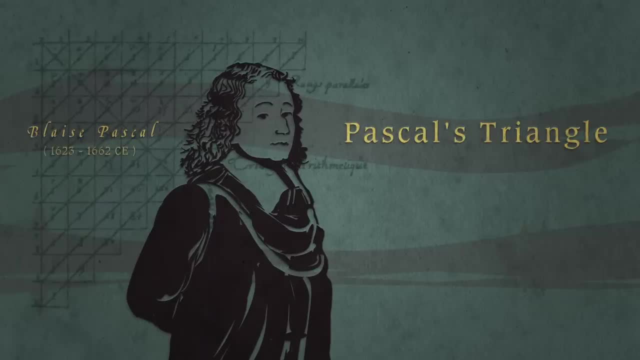 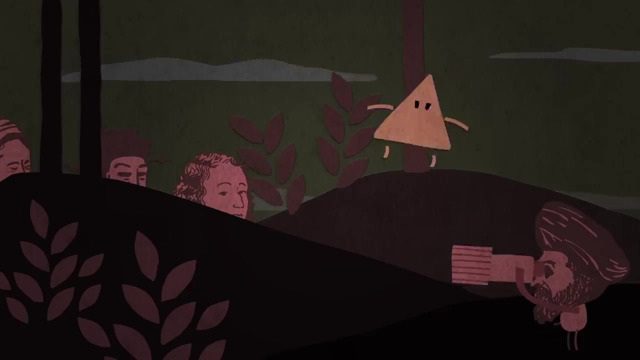 To much of the Western world it's known as Pascal's Triangle, after French mathematician Blaise Pascal, which seems a bit unfair, since he was clearly late to the party, but he still had a lot to contribute. So what is it about this that has so intrigued mathematicians the world over? 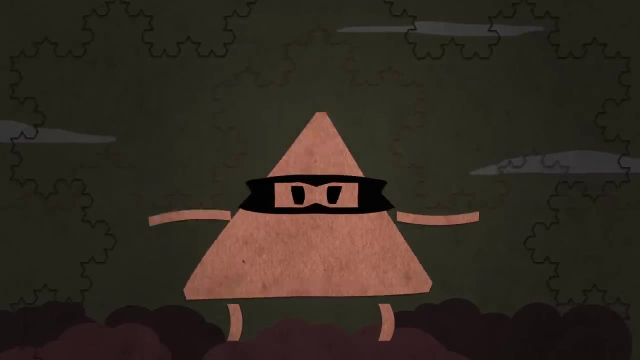 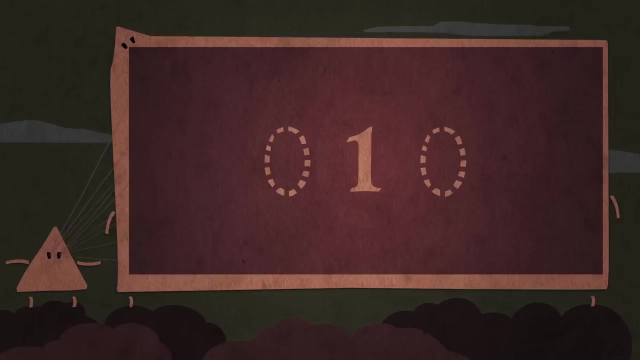 In short, it's full of patterns and secrets. First and foremost, there's the pattern that generates it. Start with one and imagine invisible zeros on either side of it. Add them together in pairs and you'll generate the next row. 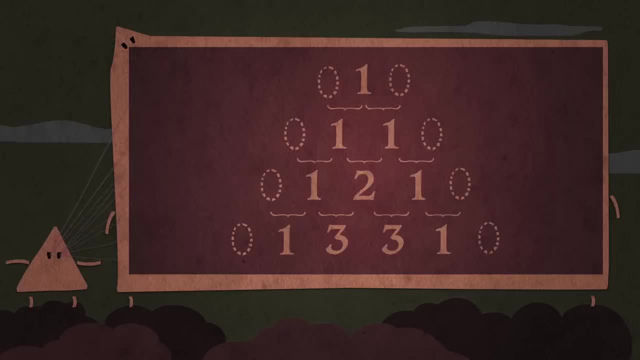 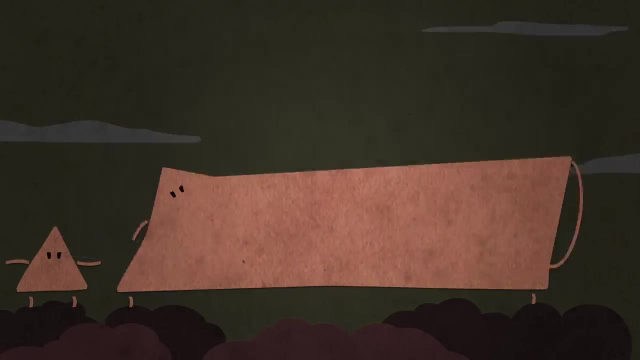 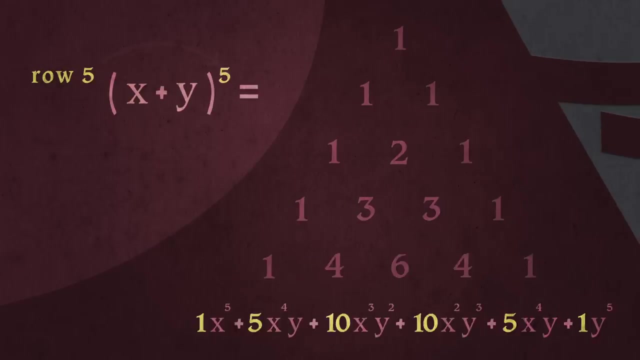 Now do that again and again, Keep going, and you'll wind up with something like this, though, really, Pascal's Triangle goes on infinitely. Now, each row corresponds to what's called the coefficients of a binomial expansion of the form x plus y raised to the n. 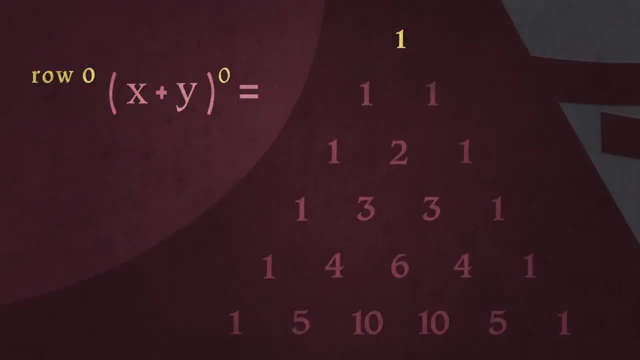 where n is the number of the row and we start counting from zero. So if you make n equal 2 and expand it, you get x squared plus 2xy plus y squared, The coefficients or numbers in front of the variables. 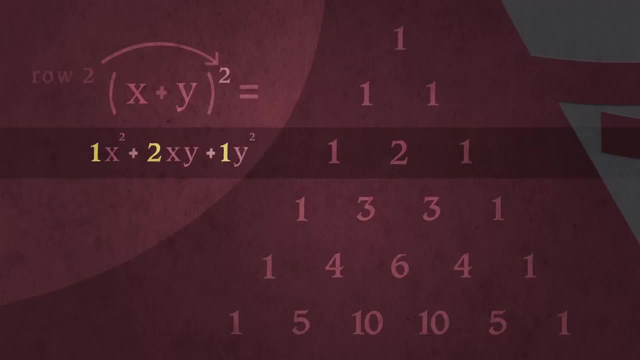 are the same as the numbers in that row of Pascal's Triangle. You'll see the same thing with n equals 3, which expands to this. So the triangle is a quick and easy way to look up all of these coefficients. But there's much more. 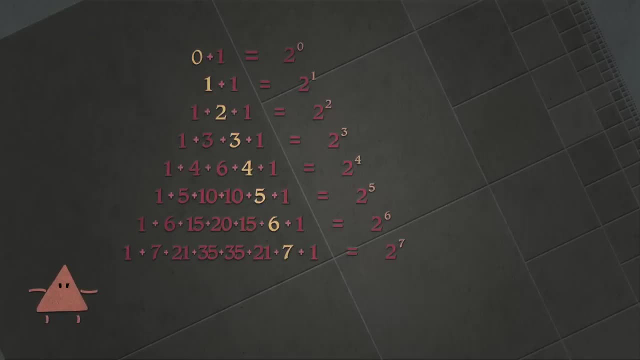 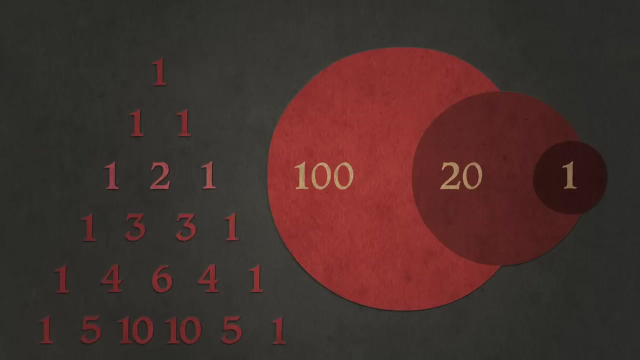 For example, add up the numbers in each row and you'll get successive powers of 2, or in a given row, treat each number as part of a decimal expansion. In other words, row 2 is 1 times 1 plus 2 times 10 plus 1 times 100.. 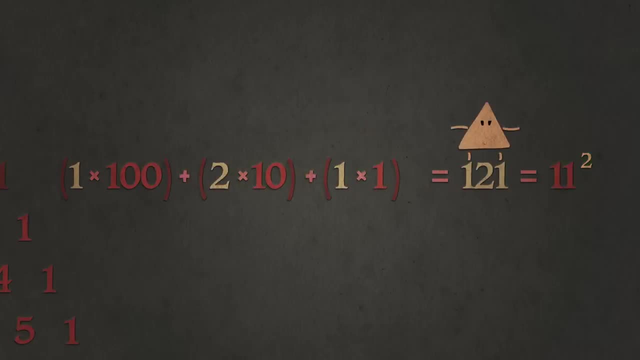 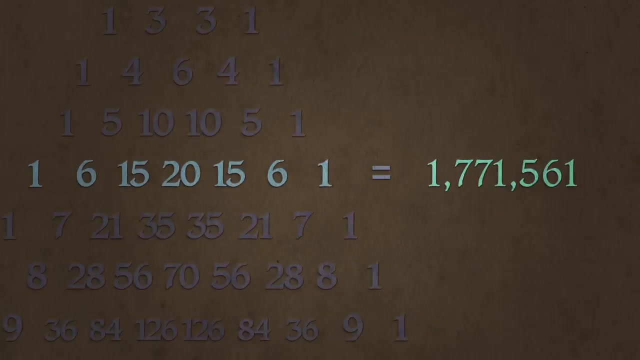 You get 121,, which is 11 squared, And take a look at what happens when you do the same thing to row 6.. It adds up to 1,771,561, which is 11 to the 6th, and so on. 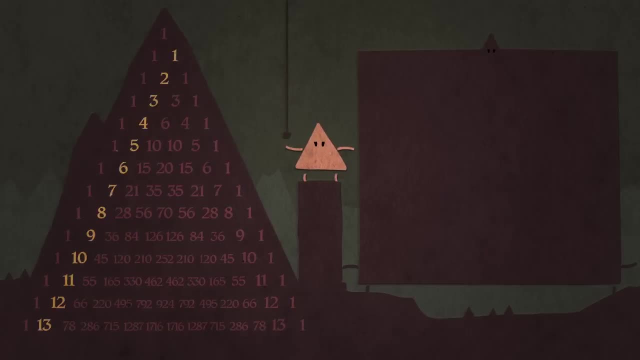 There are also geometries. There are geometric applications. Look at the diagonals. The first two aren't very interesting- All ones- and then the positive integers, also known as natural numbers. But the numbers in the next diagonal are called the triangular numbers. 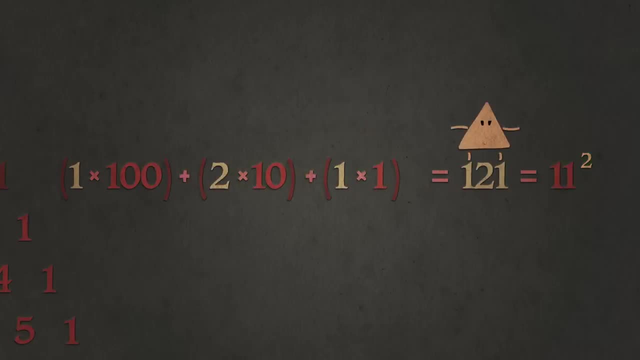 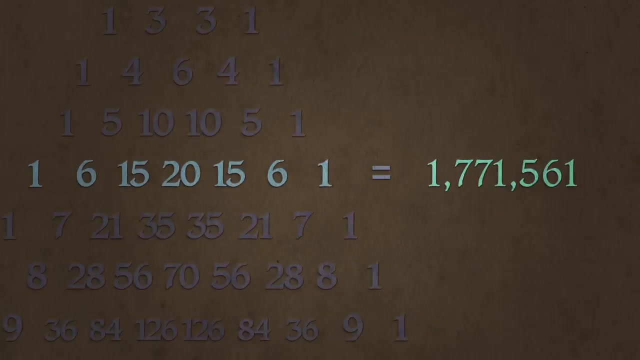 You get 121,, which is 11 squared, And take a look at what happens when you do the same thing to row 6.. It adds up to 1,771,561, which is 11 to the 6th, and so on. 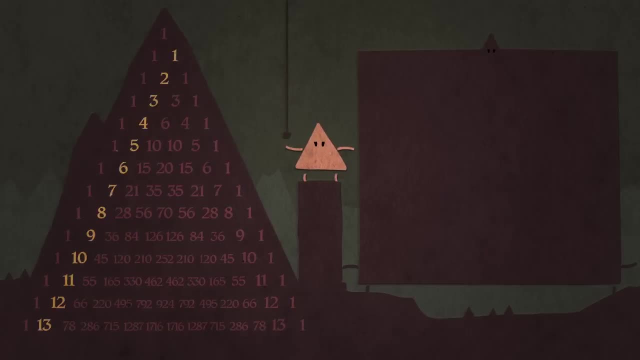 There are also geometries. There are geometric applications. Look at the diagonals. The first two aren't very interesting- All ones- and then the positive integers, also known as natural numbers. But the numbers in the next diagonal are called the triangular numbers. 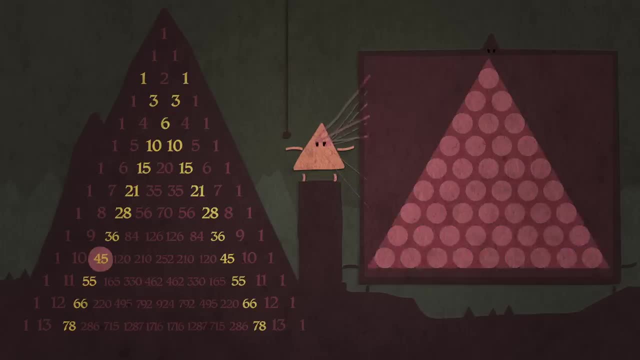 because if you take that many dots, you can stack them into equilateral triangles. The next diagonal has the tetrahedral numbers, because, similarly, you can stack that many spheres into tetrahedra. Or how about this Shade in all of the odd numbers? 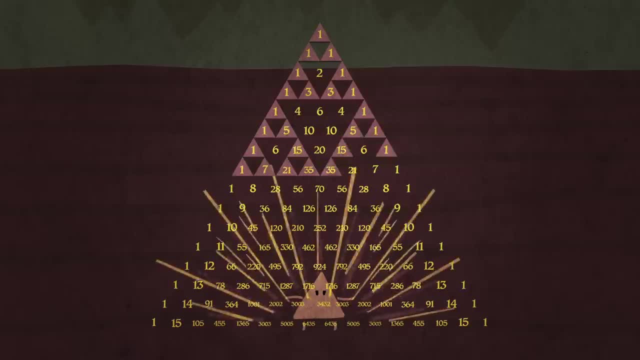 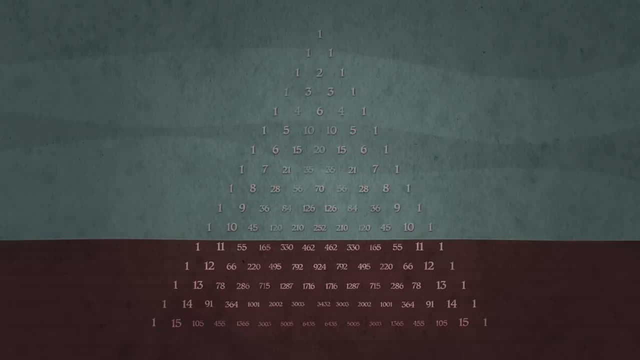 It doesn't look like much when the triangle's small, But if you add thousands of rows you get a fractal known as Sierpinski's triangle. This triangle isn't just a mathematical work of art, It's also quite useful, especially when it comes to probability and calculations. 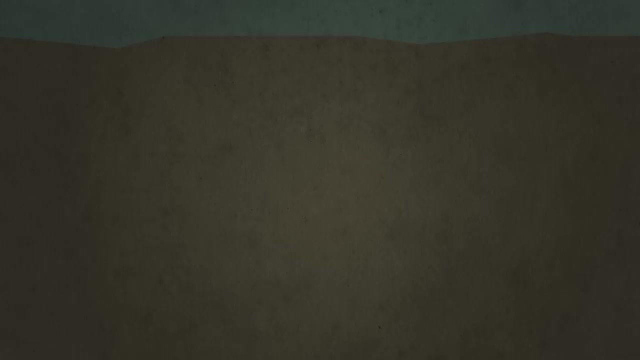 in the domain of combinatorics. Say you want to have five children and would like to know the probability of having your dream family of three girls and two boys In the binomial expansion that corresponds to girl plus boy to the fifth power. 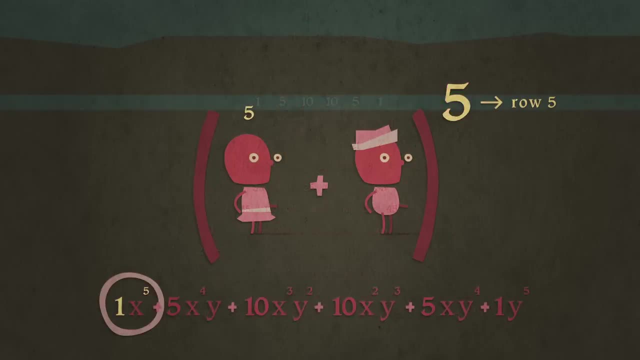 So we look at the row five, where the first number corresponds to five girls and the last corresponds to five boys. The third number is what we're looking for: 10 out of the sum of all the possibilities in the row. So 10 over 32, or 31.25%. 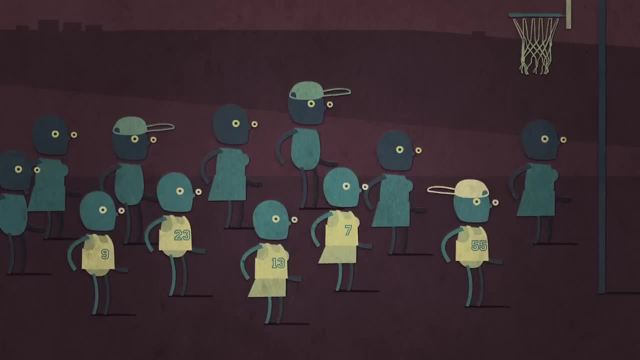 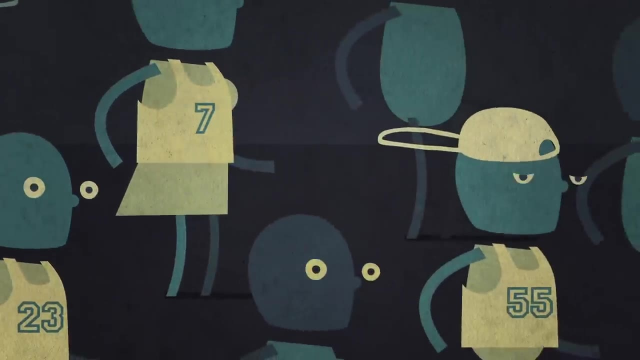 Or if you're randomly picking a five-player basketball team out of a group of kids or 12 friends, how many possible groups of five are there? In combinatoric terms, this problem would be phrased as 12 choose 5,. 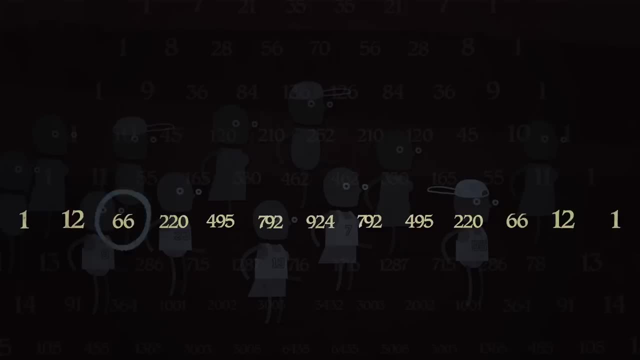 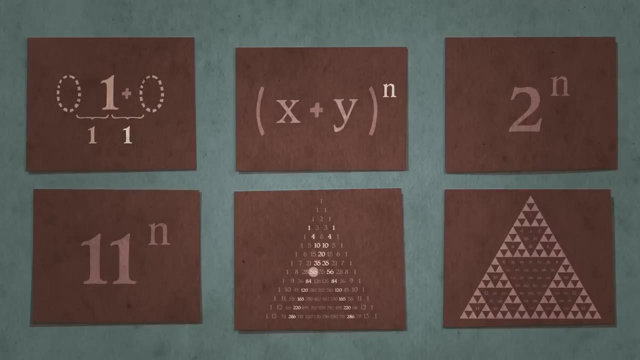 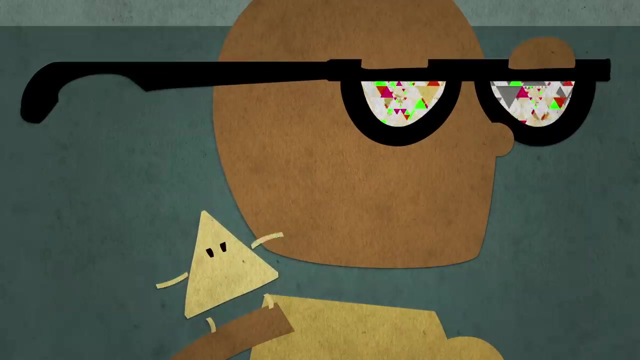 and could be calculated with this formula. Or you could just look at the sixth element of row 12 on the triangle and get your answer. The patterns in Pascal's triangle are a testament to the elegantly interwoven fabric of mathematics, And it's still revealing fresh secrets to this day.